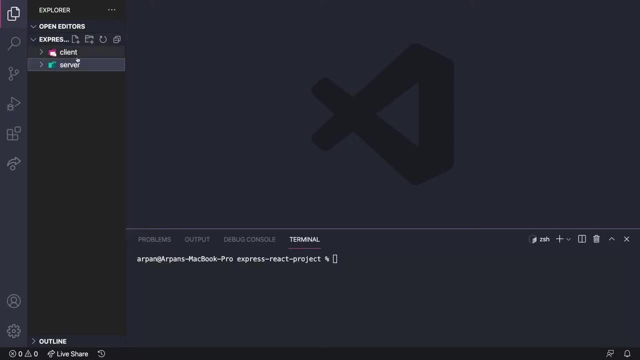 and the other one will be called server. This client directory will contain our React code and this server directory will be where we write all of our Express inside of. So this backend is the server folder and the client is our frontend. Next we can move on to setting up our project files. So I'm going to first set up our 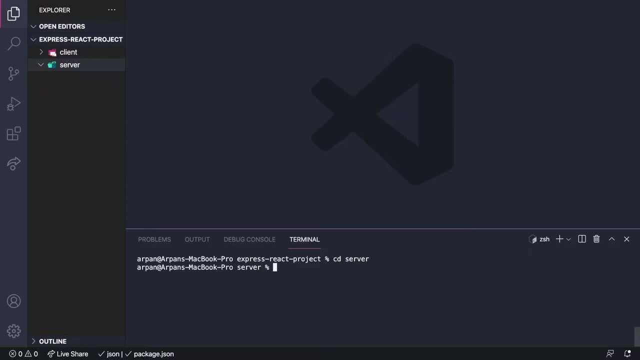 files in the server. So I'm just going to cd into the server directory and then run anything. So I'm going to cd npm init, hyphen y, to answer yes to all the questions and to generate a packagejson file that you see right here. And then here I'm going to change my server's. 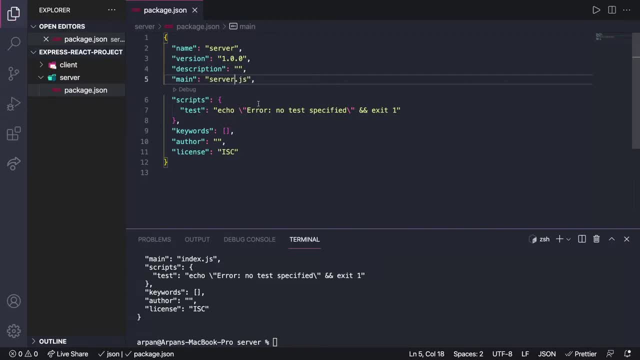 file name to serverjs. If you want to keep it at index, you can, but I just prefer the name serverjs. so I'm going to rename it to serverjs and I'm also going to create a serverjs file. So touch serverjs, and I'm also going to install Express, So I'm 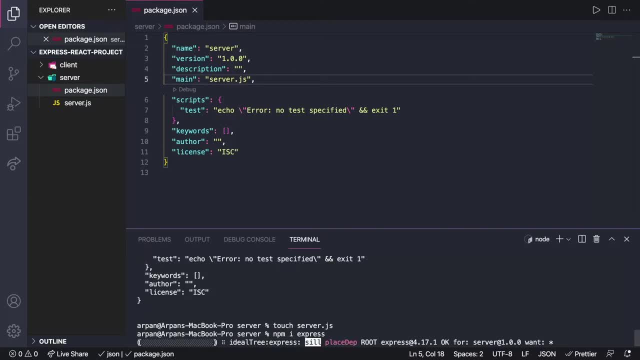 going to do npm i- express, And then I'm going to install nodemon so that if we make any changes within our server file it will automatically restart the server. So I'm just going to do npm i- nodemon and then I'm going to do hyphen capital D to basically note that it's a dev dependency. So it's. 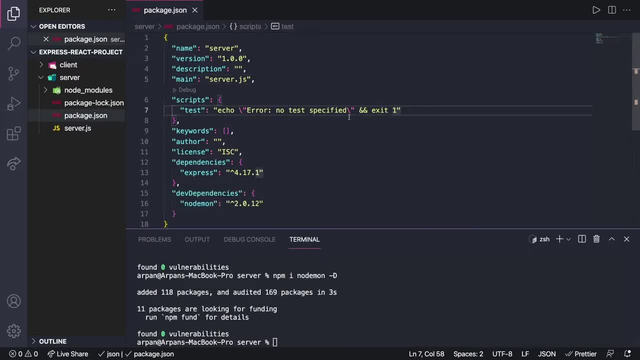 going to install nodemon And then in our scripts I'm going to create a script to start up our server. So start is going to be node serverjson, And then I'm going to put dev for nodemon server And you'll understand this once we. 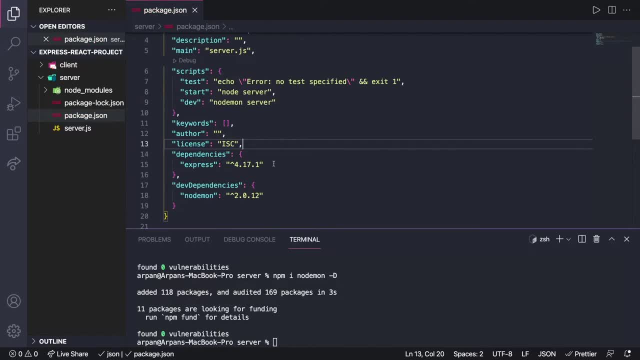 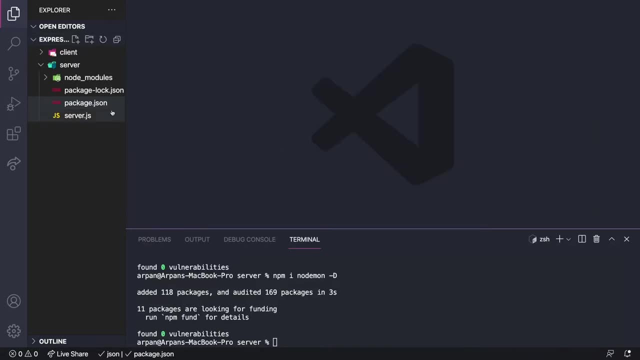 start up our server file, And so right now we've installed Express and nodemon, and this is all we need for right now. We'll install packages later on if we need them. So now that we have our server configuration done, we can move on to the client configuration. 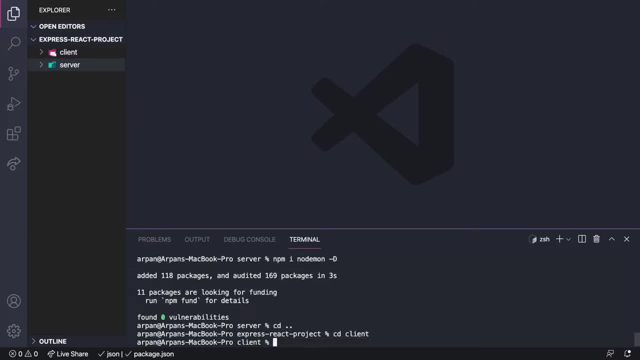 So I'm just going to cd out of this directory and then cd into client And then here what I'm going to do is just create a react project. So I'll just do npx- create clientjson- Create react app and I'm going to do dot to create it in the client directory And 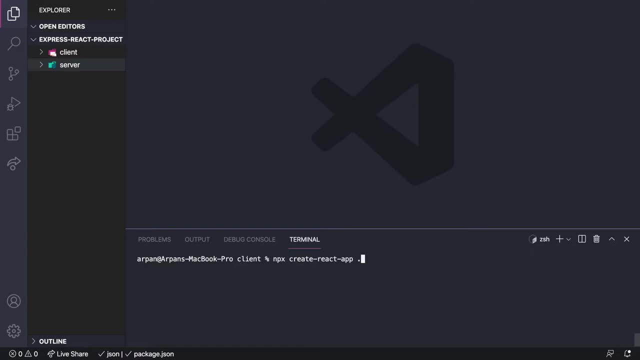 this process will take a while, so I'll cut back to the video once the react project has been created. Alright, so now that our client project has been created, I'm just going to go on into this client directory source and then I'm just going to remove all the boilerplate code. 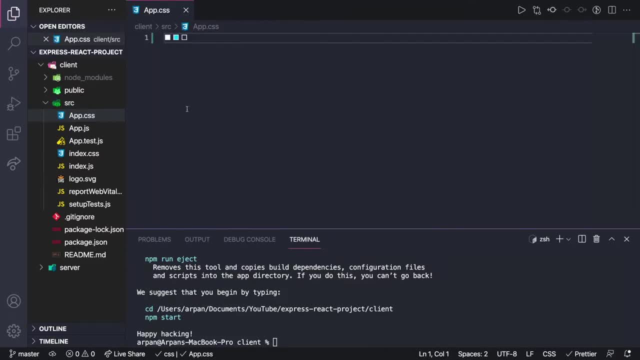 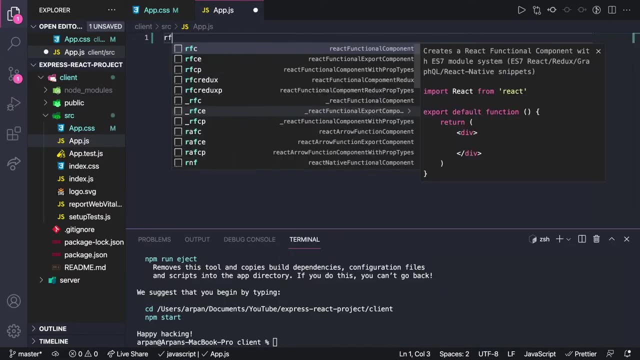 So I'm just going to remove everything in appcss and then I'm going to remove everything in appjs and I'm just going to replace it with a normal functional component. So I'm going to do rfce so that we get a functional component like this, And now that we have 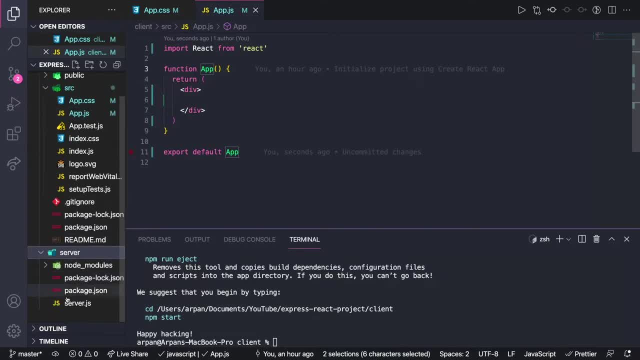 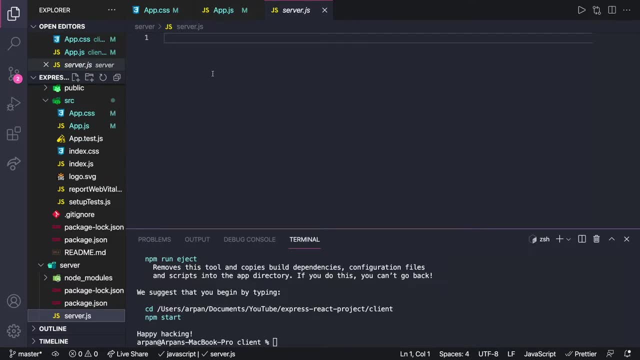 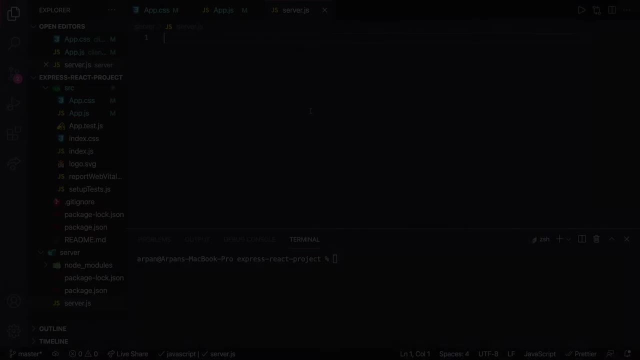 this setup, we can start setting up the backend API in our serverjs file. So we're going to set up the backend API first and then start our server and then move on to displaying the data from the backend onto the frontend in this appjs file. 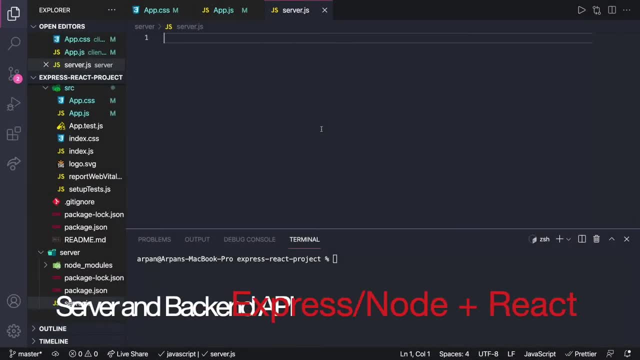 Now, to set up our backend, we're going to need to import express first, So I'm just going to do constjson- Express is equal to require express. And then, in order to create our app, I'm just going to do const- app is equal to express, And I'm going to set up a route for the API, So I'm 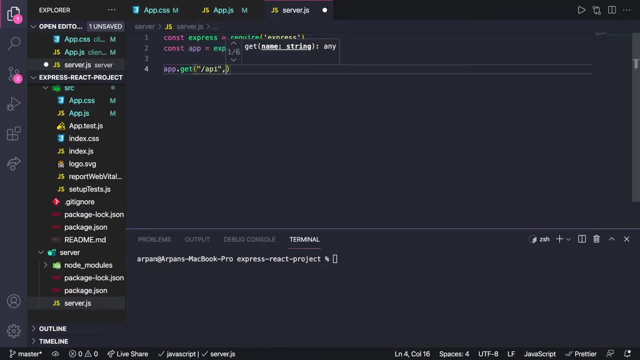 just going to do appget forward slash API and then request and response, And then here I'm just going to send a JSON array of users. So I'm just going to do resjson And then do users And this will be equal to an array of users, basically. So I'm just 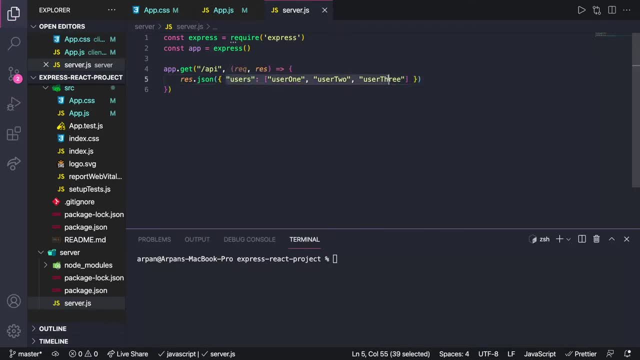 going to do user1,, user2,, user3.. Alright, and this is basically our backend API, right here And in the frontend, what we're going to do is basically fetch this users array and display every single user. OK, and in order to start up our backend, I'm going to do applistenappapp. These are usually fairly common高 needs. Anyways, we're just going to start this up and then that future will show up automatically. So we're just going to set that Now, if you'd like to show it to the right color. So I'm just going to do. you're going to show that data shade and 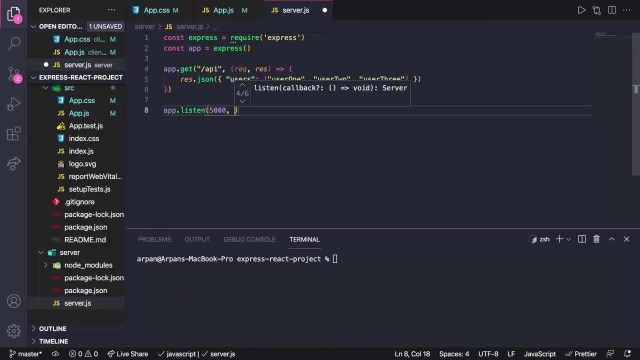 at port 5000.. Alright, so the server is going to be running on port 5000 and the client is going to be running on port 3000, because react by default runs on port 3000.. And then, once the server is listening on port 5000, we're going to need some sort of message to tell us that it's 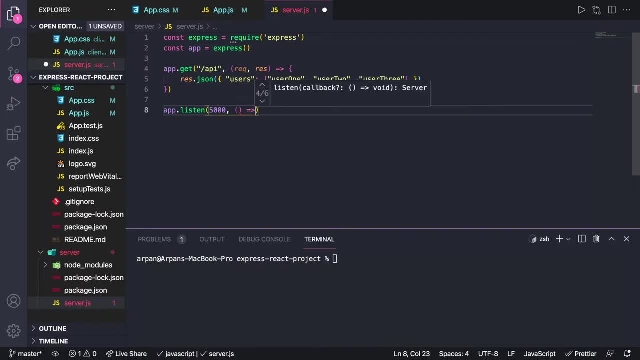 listening on 5000.. So we're just going to do an arrow function and this will just have consolelog server started on port 5000.. Okay, and then to start up our server, I'm going to go into the server directory and I'm going to run npm, run dev and the reason that we're going to need to do npm. 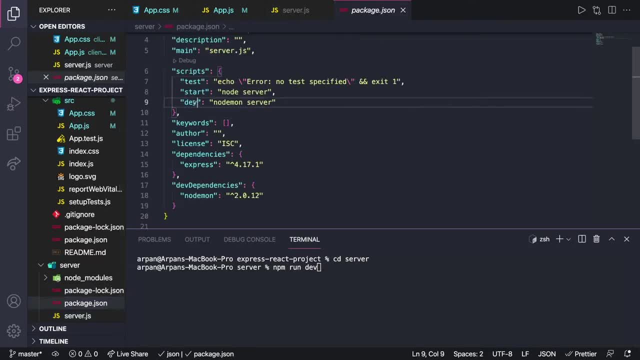 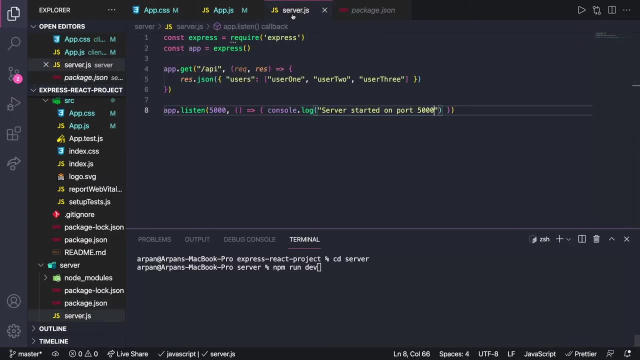 run dev is because in our packagejson this dev right here, we'll call nodemon server, Alright, so when we run this it'll start up the server with nodemon. So if we need to add anything else, we're going to do that. So we're going to do that. So we're going to do that. So we're going to do. 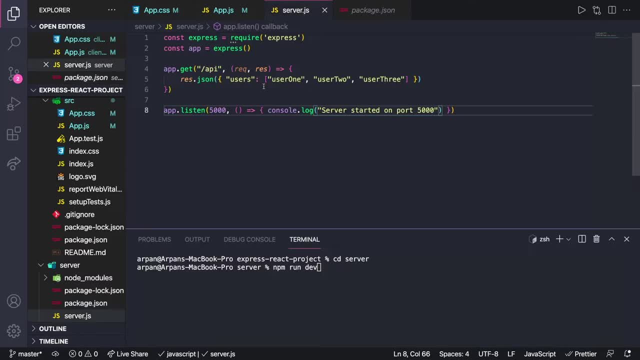 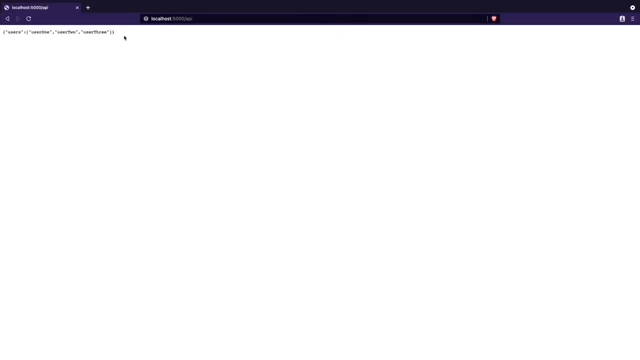 the server will automatically restart and we don't have to do it manually. So I'm going to hit enter and right here you can see that it says server started on port 5000.. So if we go to our browser and type in localhost, port 5000, forward slash api, you can see that it has returned the. 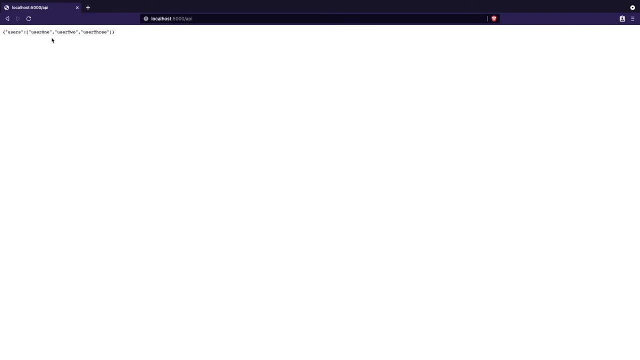 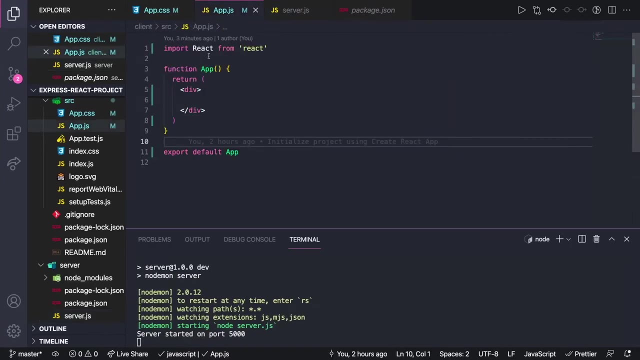 json data right here of the user's array with user one, two and three And next. we just need to display these users onto the front end with this appjson And to display these users we're just going to use use effect to fetch the api and then to you know. 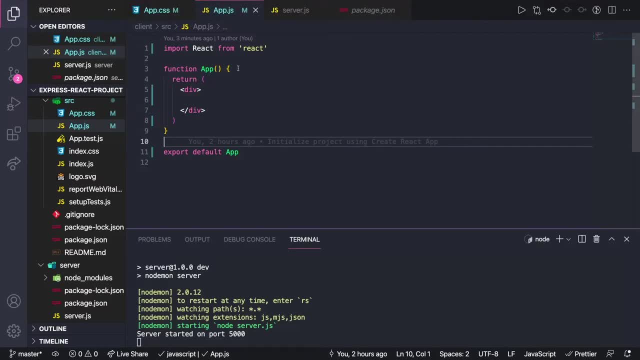 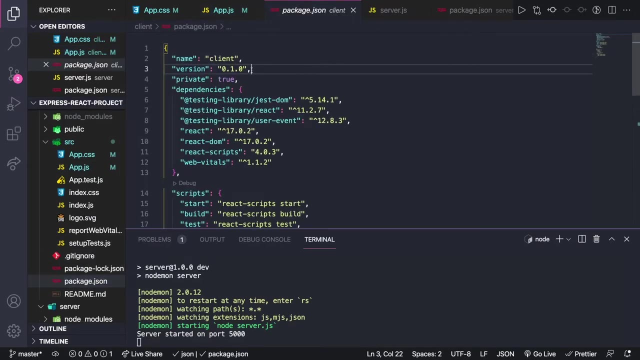 have these users, we're going to have them stored inside of a variable and then use that variable to display the users on the front end. Now to get started with the front end, I'm going to open up the packagejson file that you see right here in the front end, Alright, and I'm going to create a. 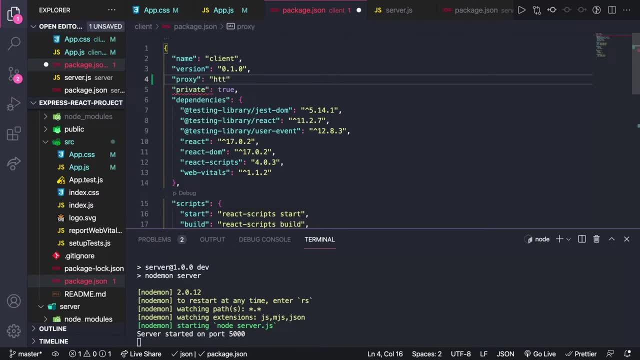 line called proxy and this will be set to http localhost port 5000.. Okay, and we're putting this line so that we can make relative api requests and also avoid any issues that we might run into with cross origin. So next in our appjs, I'm going to 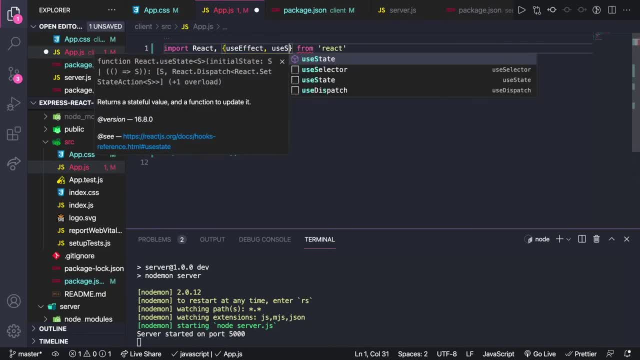 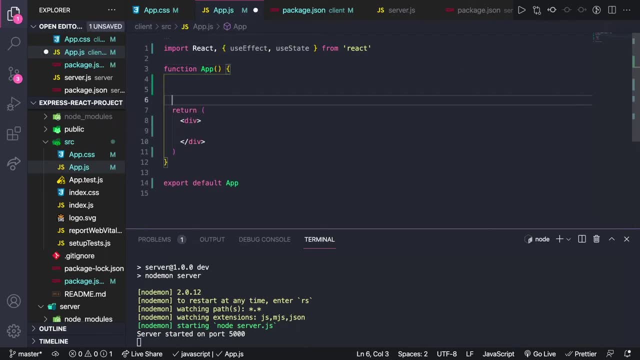 import use effect and use state. Alright, and if you don't know what these two are, I have videos on them which will be on the top right hand corner of the screen. And next, I'm going to create a state variable which will contain the back end data that we 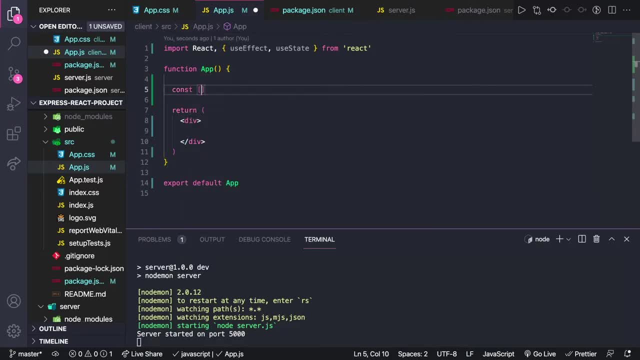 get from the back end api. So I'm just going to do const back end data, set back end data and this will be equal to use state. Okay. and then next we're going to fetch this back end api And to do this I'm just 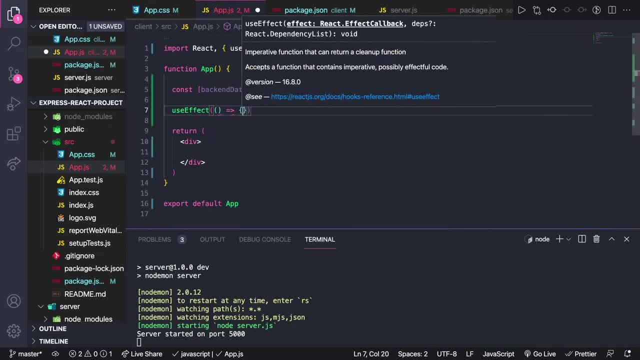 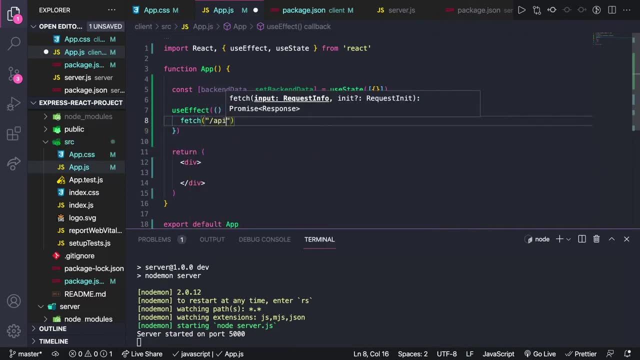 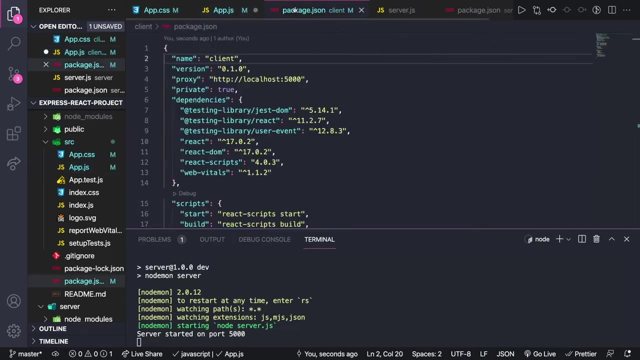 going to do use effect and then the effect will basically be a fetch api. So I'm just going to do fetch forward slash api and we're just going to have the. we can just put the relative route instead of putting in localhost 5000, since we've defined this proxy in our package: dot json. 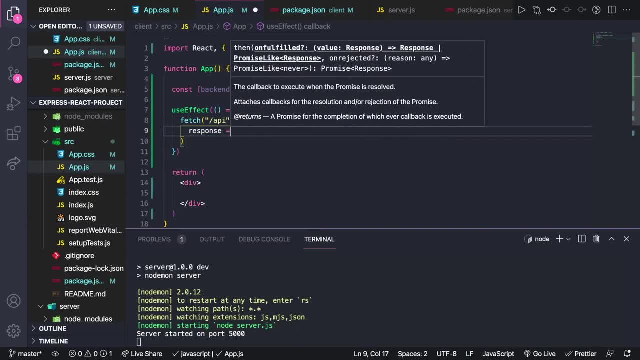 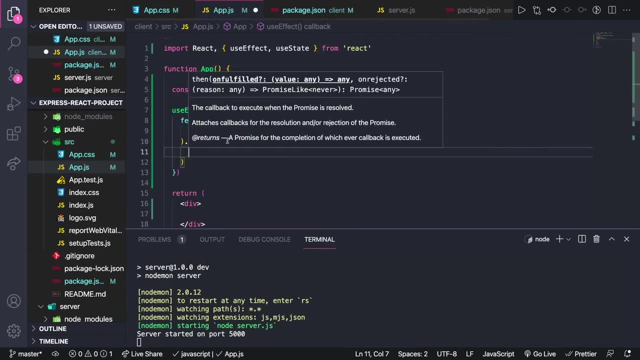 Okay, and once we fetch the api, whatever response that we get from the api, we're going to get the response in json And then, once we get the response in json, we're going to basically get the data inside the json and set that data to this back end data variable right here. So we're going to actually set that data inside the json and set that data to this back end data variable right here. 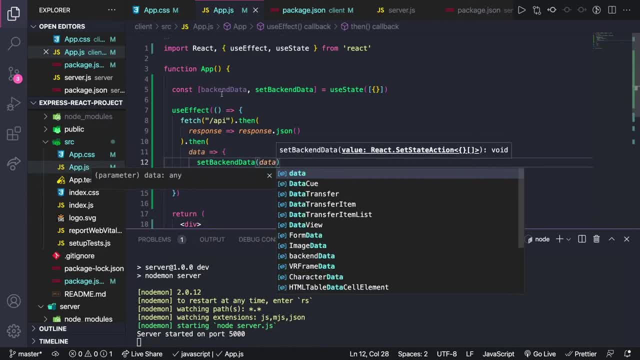 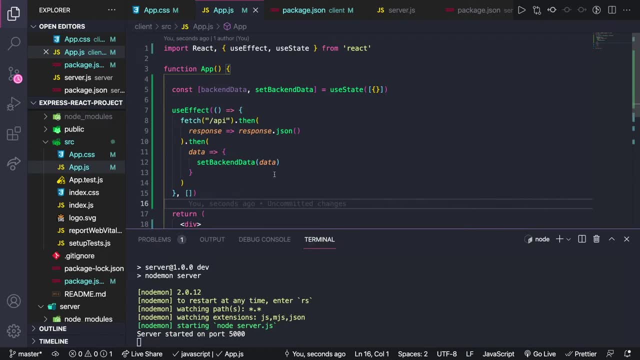 So I'm just going to do set backend data to data, and I'm also going to pass in an empty array so that this only runs on the first render of the component. Next, we need to start up our frontend, so I'm just going to open up another terminal. 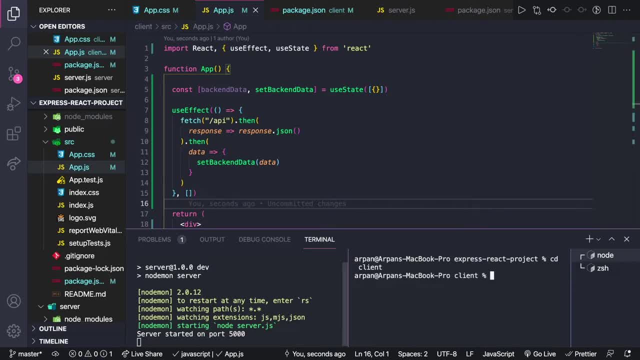 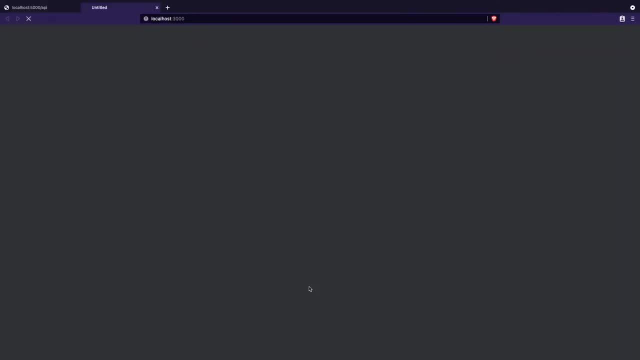 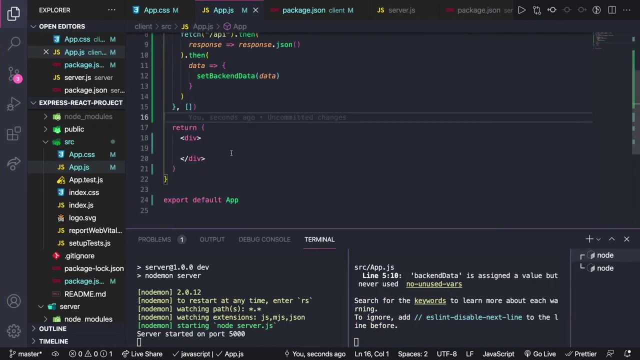 window and then go into client, so cd client and then npm start. This will start up the frontend on localhost port 3000, so just give it a couple of seconds and you can see that it's loading up And there's nothing on the page and that's because we have nothing rendered over here. 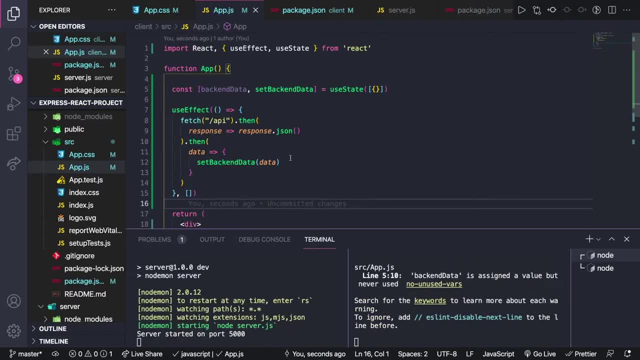 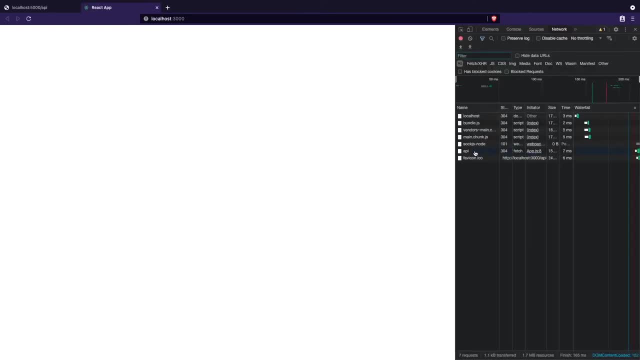 but it should have fetched this API and to check if it did fetch the API or not, we can just open up the network pane right here and then reload it and you can see that there was a fetch request sent to the backend API and you can see that it has the users right. 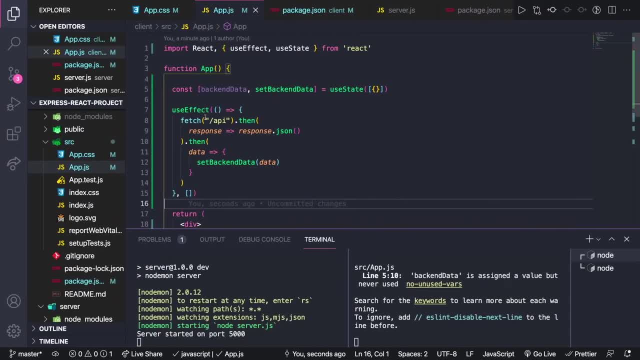 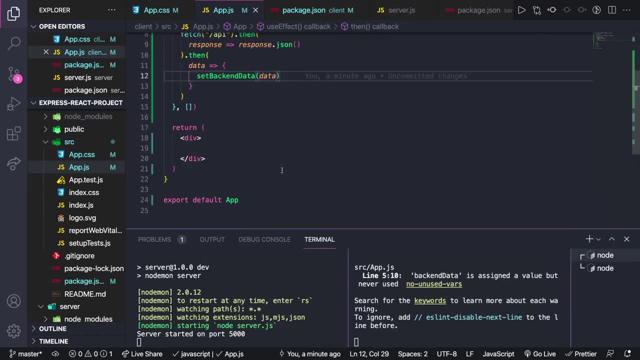 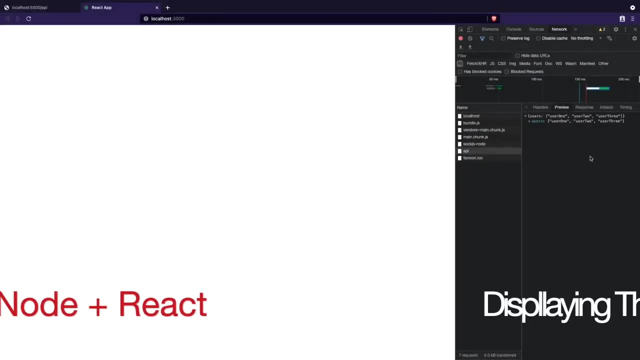 here. So we know that this API fetching is working with useEffect and it's setting the data to this backend And the next step is to just render the users onto the webpage. Okay, so now that we see these users here, we know that the API fetching is working and 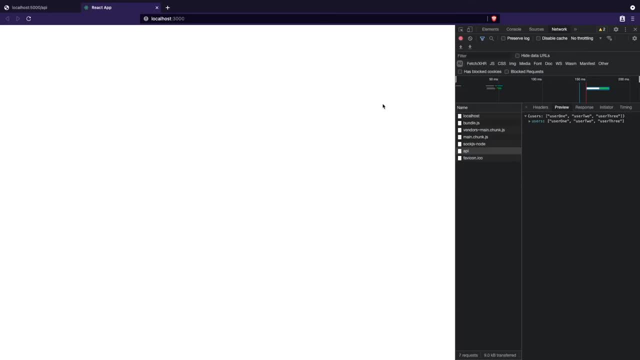 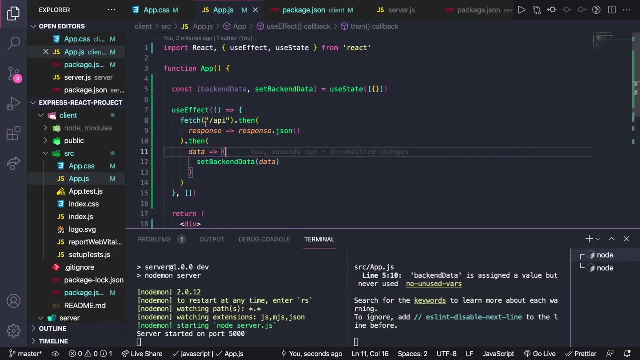 we're done with fetching APIs and we just need to display the users onto the webpage, but I just want to go a little bit deeper as to how this useEffect works. So, basically, what it's doing is fetching this forward slash API route, which is actually 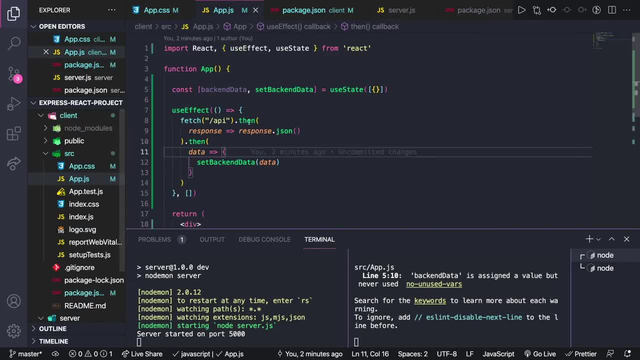 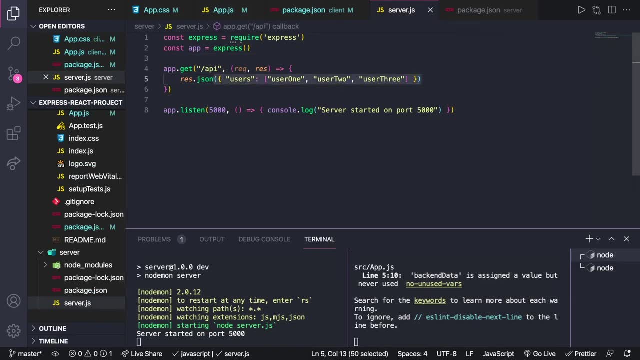 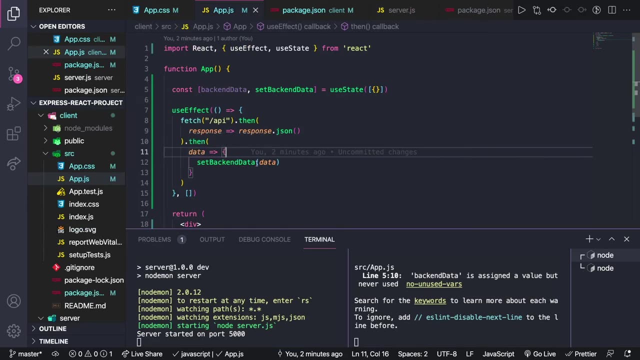 this API route in the backend And whatever response that it gets after sending a GET request to the API will be this response. you see, right here, This JSON is the response that the client will receive and then, whatever data is in that JSON, we're going to set that data to this backend data variable. 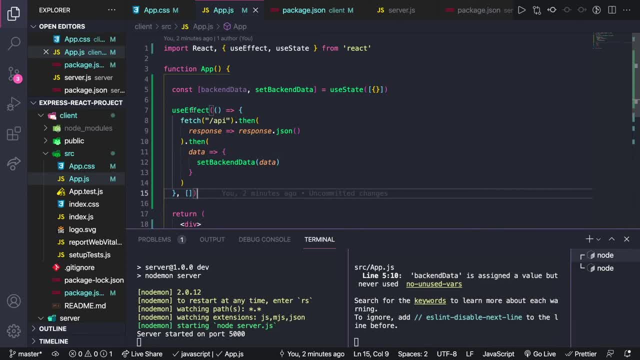 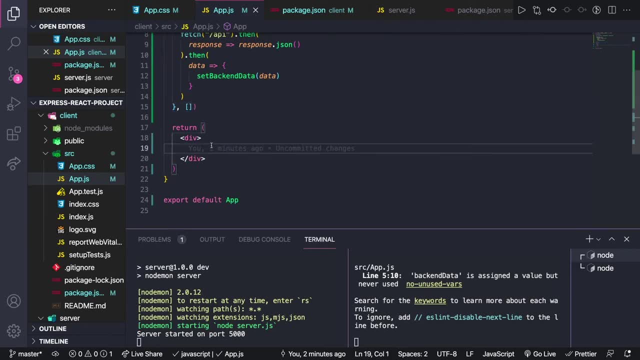 And I've just passed in this empty array at the end so that this useEffect block only runs on the first render of the component. Okay, Okay. Next, we just need to display the users. So to display them, I'm just going to write down some code and I'll explain along the 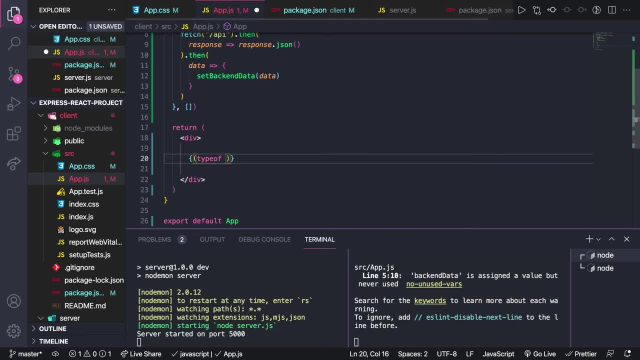 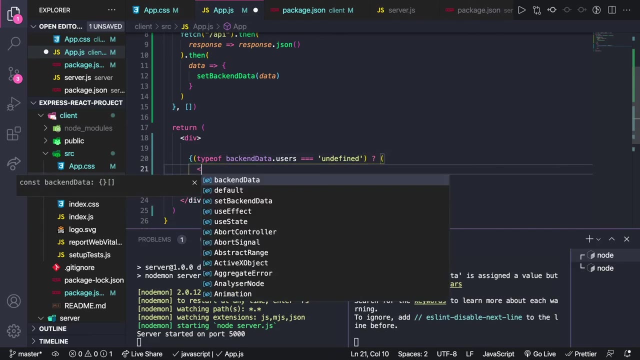 way what it means. So I'm going to do. if type of backend datausers is equal to undefined, meaning that we haven't gotten the users yet, or the API is currently being fetched. we're just going to display loading Otherwise meaning that the API has been fetched. 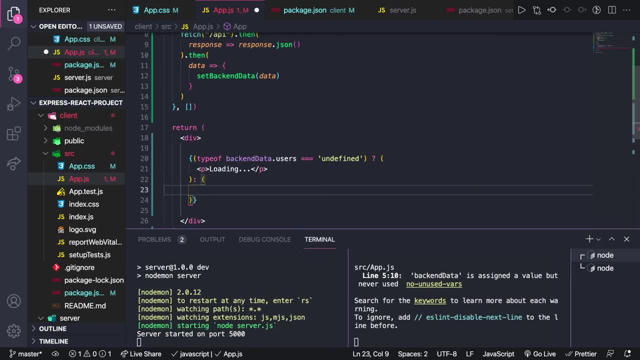 Okay. So now that the API has been fetched and we have the users, we're basically going to map them to a p tag and display them. So to display them, I'm just going to do backend datausersmap user and then i which is going. 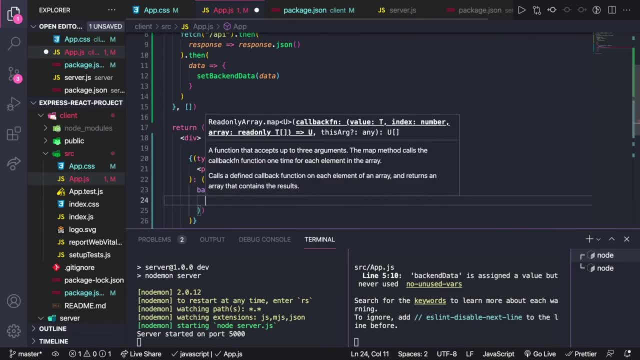 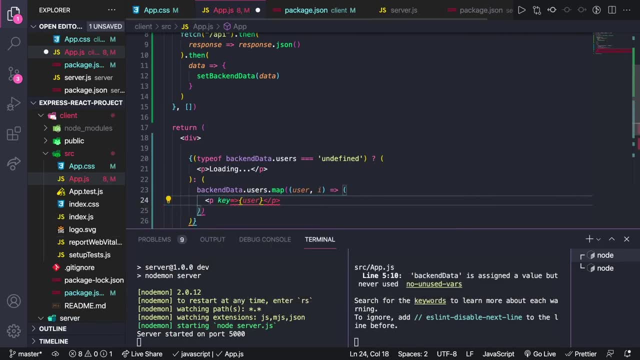 to be the key for each p tag. We're basically going to display them by doing p and then user and key will be i. Okay. So if we go here, you can see that it has rendered user one, two and three. 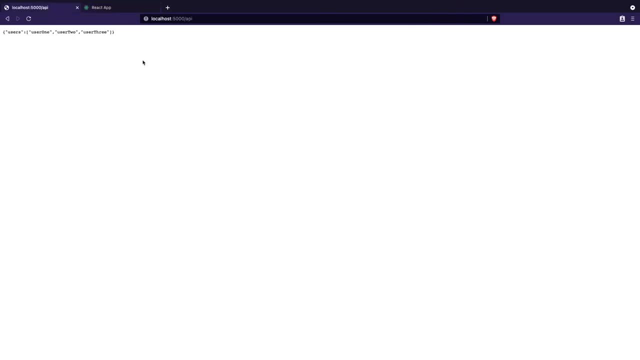 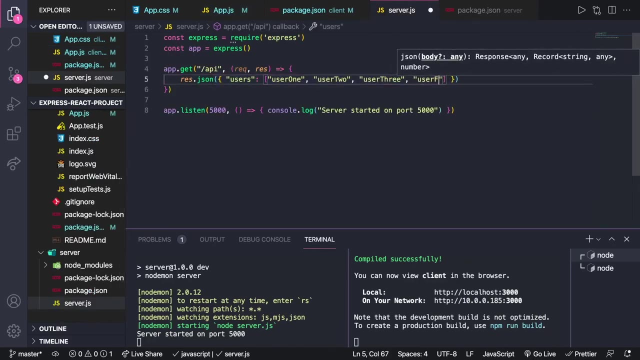 Okay. So if we go here you can see that it has rendered user one, two and three from the backend. Now if we add another user to the backend, let's say we want to make user four, So user four all right- and then refresh this. 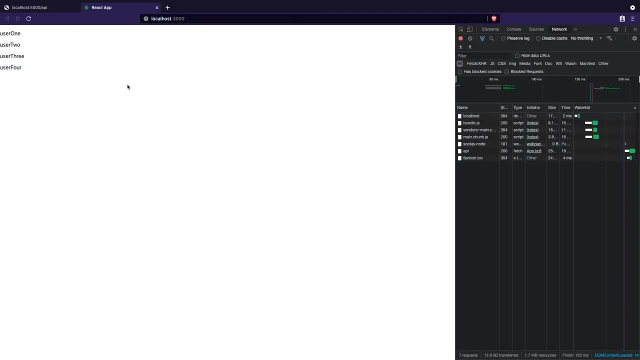 You can see that it has user four. So this is basically our app and we're basically done with it. All right. So now that we're done with this app, I just want to recap on what we did. So first, we created this backend server with express. 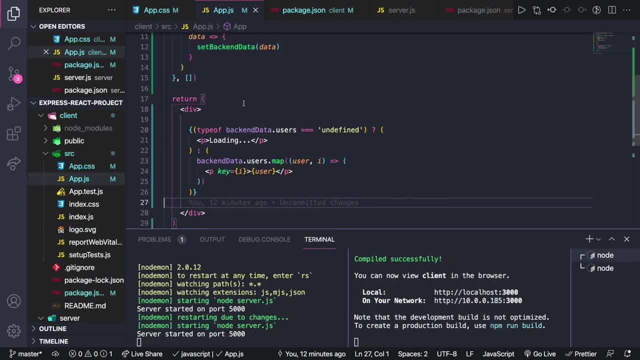 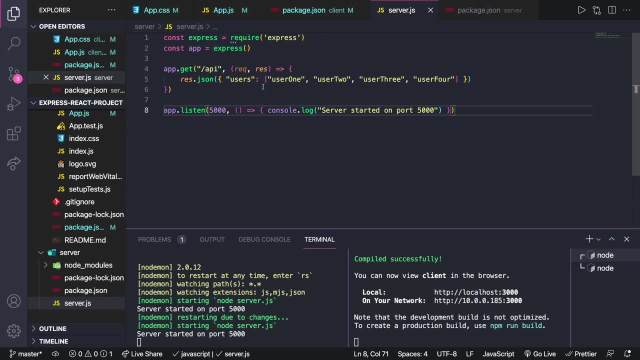 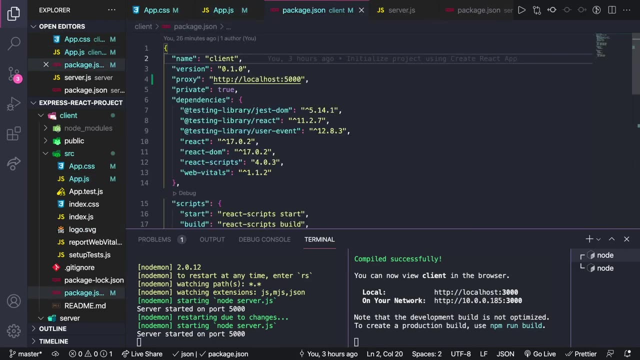 Okay, It's frontend with react, right, And in our backend we set up a backend API that returns a list of users And what we wanted to do was show those users on the frontend, which is in react, And to show them on the frontend, we first set up a proxy in our packagejson file in. 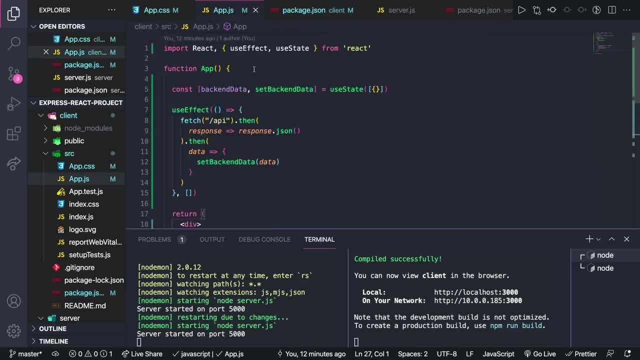 the frontend and then used the use effect hook to fetch the API and then store the data that the backend returned using the use state hook inside of this backend data variable. Okay, So now that we have the data, we first check if the data has been retrieved or not. 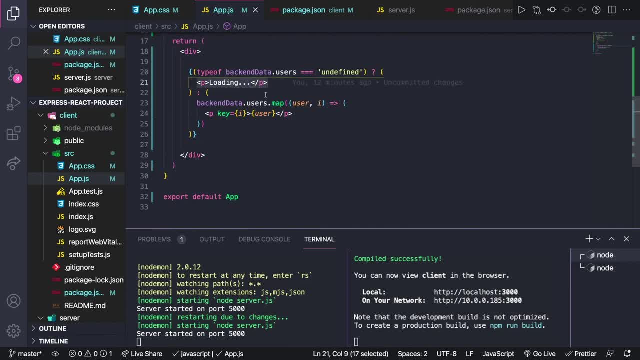 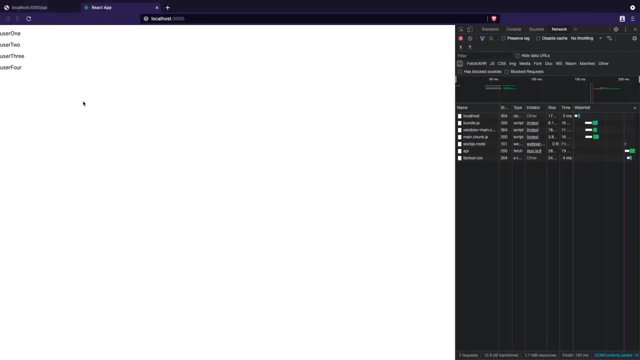 And if it hasn't been retrieved, we just display loading Otherwise, meaning that it has been retrieved. we map each user to a P tag and display them like this. So yeah, that's basically it for this video. I hope you enjoyed and learned something. 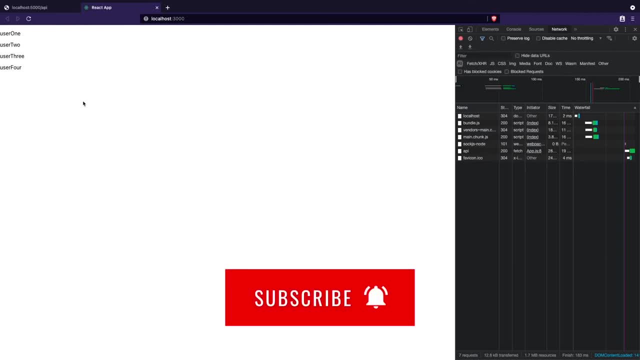 And if you did make sure to leave a like and subscribe to the channel for more videos like this and turn post notifications on to get notified when I upload, And I've also encouraged you to add more to this. So let's say you want to make an app. 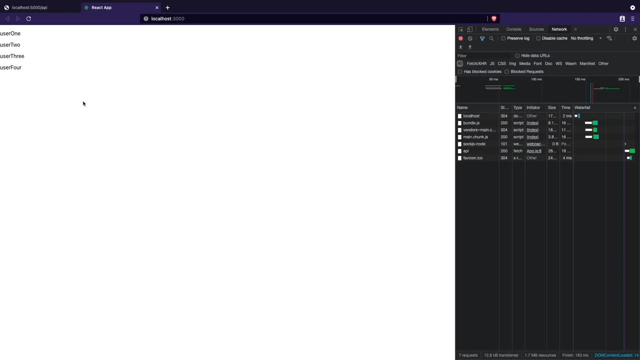 Where you can. you know post pictures. You can use Axios with React to send post requests to the backend and you know handle those post requests and you know save that picture to a database or something like that. So yeah, there's many other things you can do with this as well. 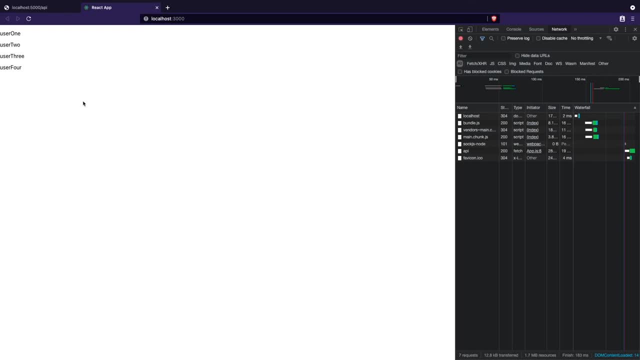 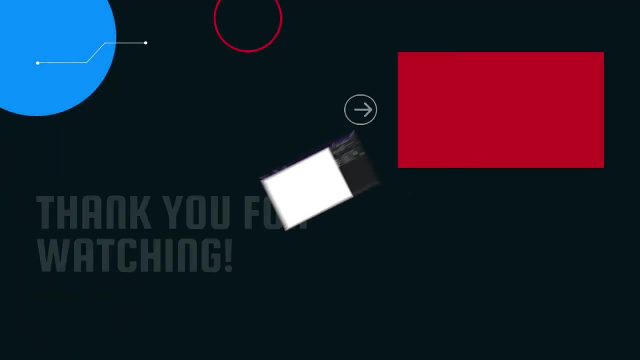 And this video is mainly just to help you get set up by connecting a React frontend to a Node or Express backend. So yeah, with that being said, I'll see you in the next video. Bye, Bye.